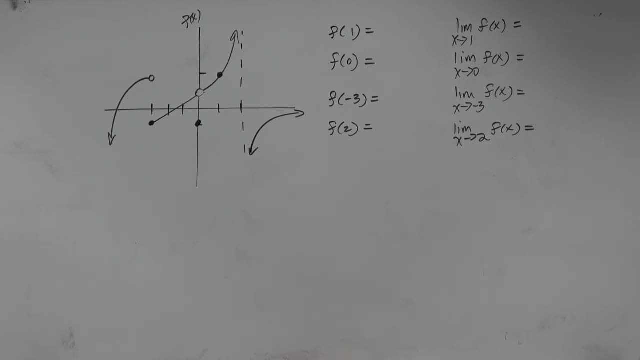 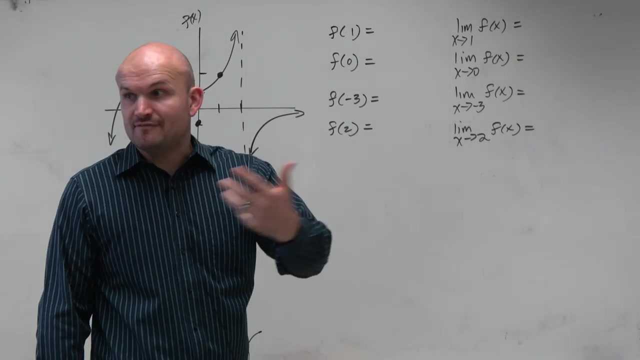 So if I was given this graph- and let's just kind of do one by one- If I said what is f of one, That means we're looking for the value of the function at f of one. So we go to one and we. 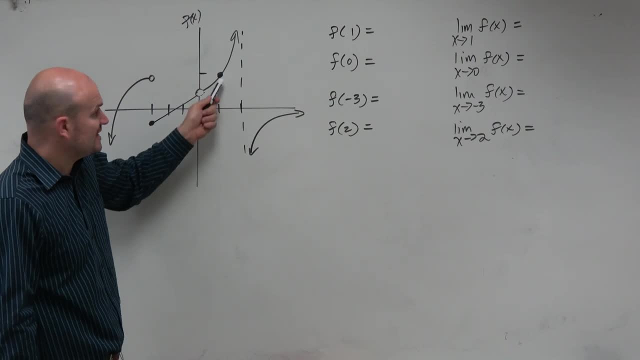 say: what is the value of the function? Well, the output value. right, That's the value of the function. So we find the y value or the f of x value, and we see that it is equal to two. So 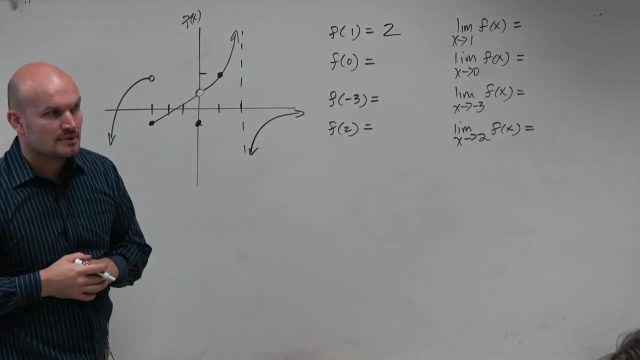 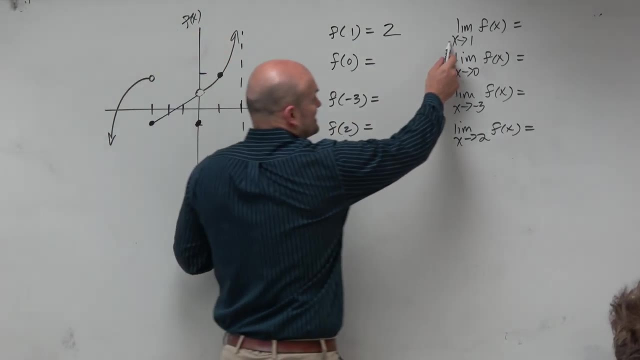 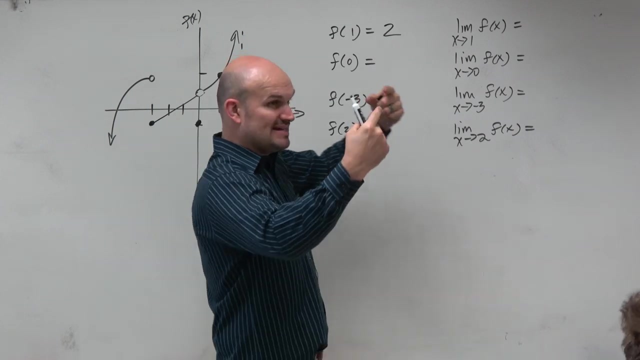 we say f of one is equal to two. Now the limit is something different. The limit is saying what is the value approaching as x gets closer to one from the left- Remember the table From the left as well as from the right. So you can basically kind of take your two fingers and kind 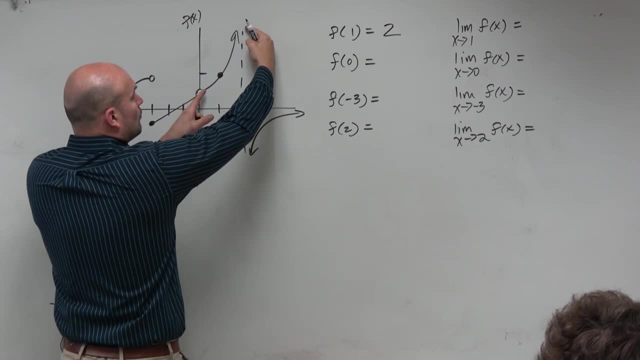 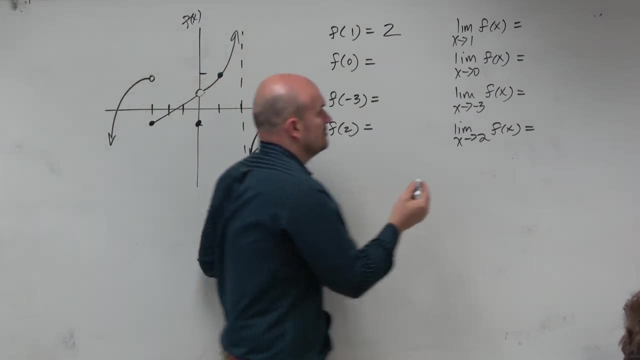 of squeeze the graph and say, all right, from the left and from the right, what y value or f of x value? am I getting closer and closer to, Or am I approaching Two? Oh okay, Well, that was easy. 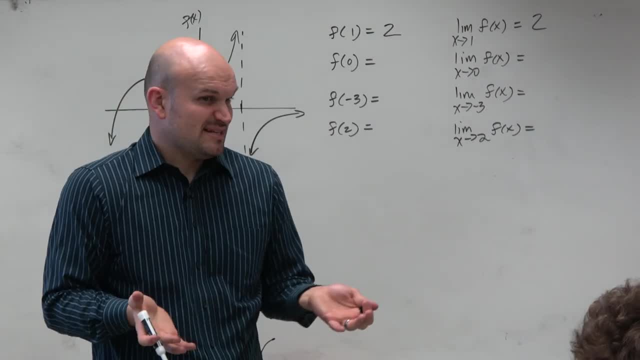 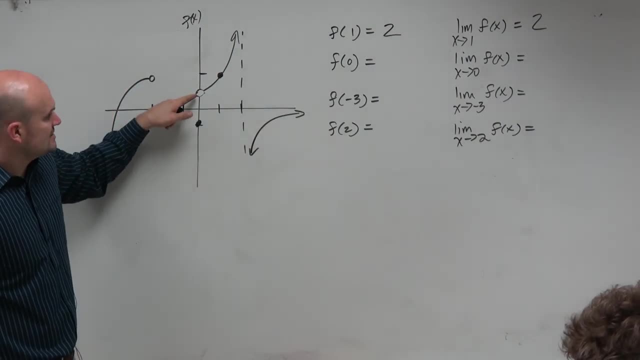 All right, I'm done. That was it. Yes, Same answer, But it's not always the case. Let's look at the next one: f of zero. We go to f of zero and we notice there's a hole. So we obviously know that it's undefined there. 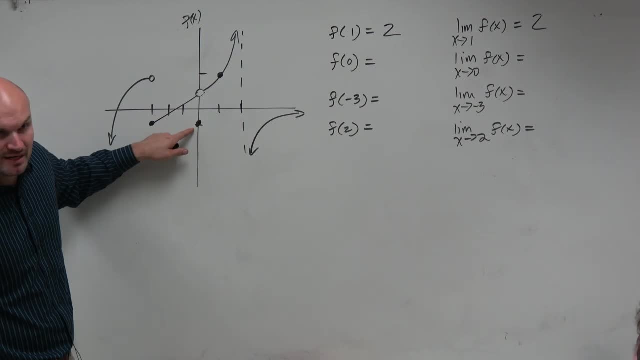 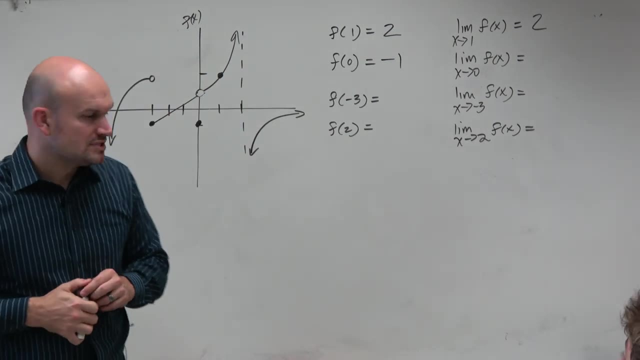 but there is a dot here that is being in replacement of that. So therefore, at f of zero is equal to negative one. So it does a jump, but then it does It's a hole. That's a hole, right, It's not available there, but it's available there, Yes, Or it could be just a. 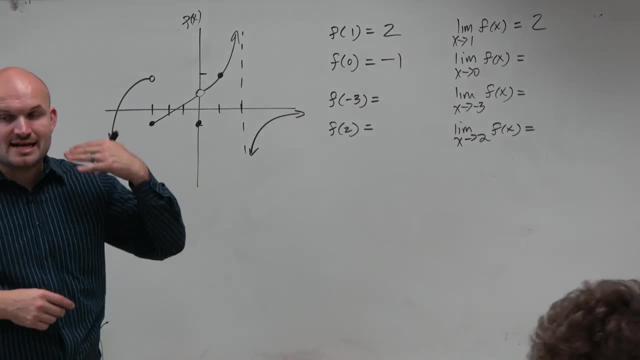 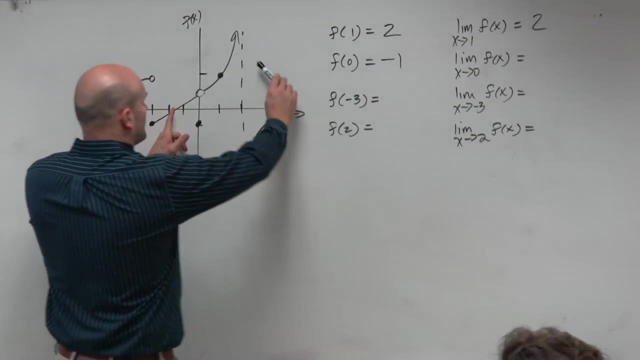 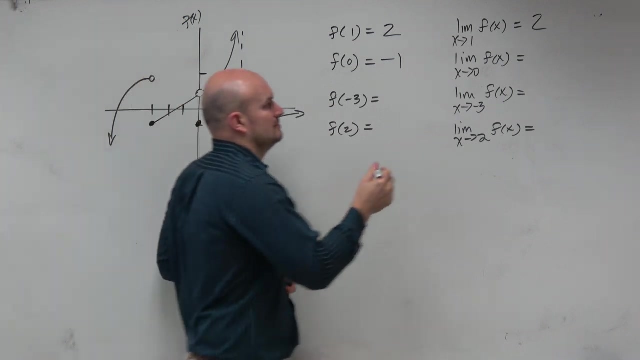 double jump, No. So now the next thing is let's answer the limit question. The limit question is saying: but then what is the value that the graph is approaching? So again, we follow our fingers here and we see that it's approaching not negative one. It's approaching what Positive one? 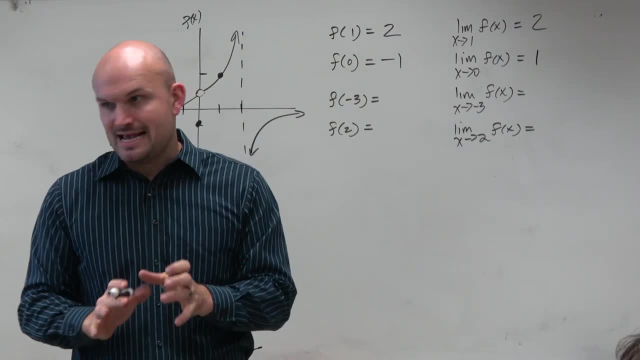 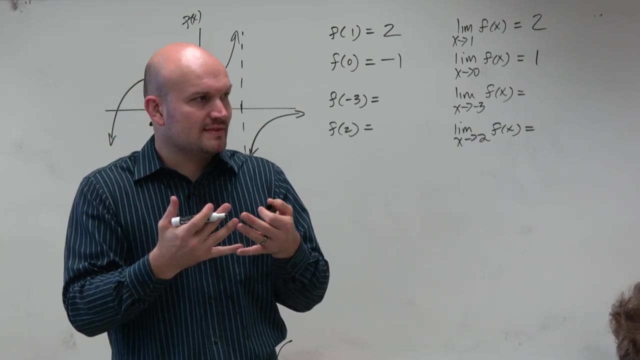 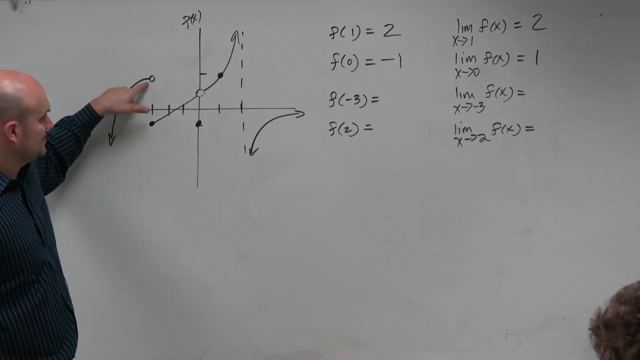 So notice these answers are different. They're not the same. The value is not the same as the limit. No, It's where it's approaching, not the actual value. Let's go and look at f of negative one, Negative three. So we go to negative three. F of negative three is not up there, That's. 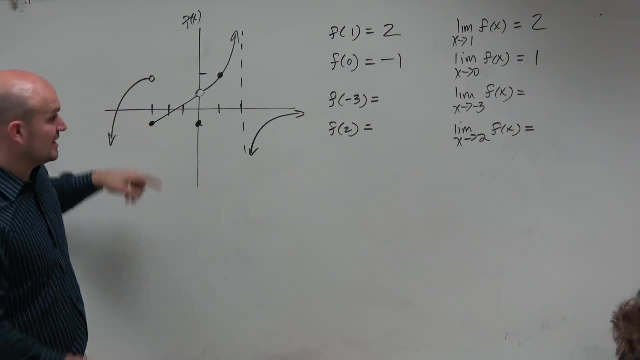 undefined. right, That's a hole. That's the filled-in line, So that's going to be also negative one. However, where is it approaching? Well, from the left, it looks like it's approaching two. From the right, it's approaching negative one. So is it approach? Can we write two?